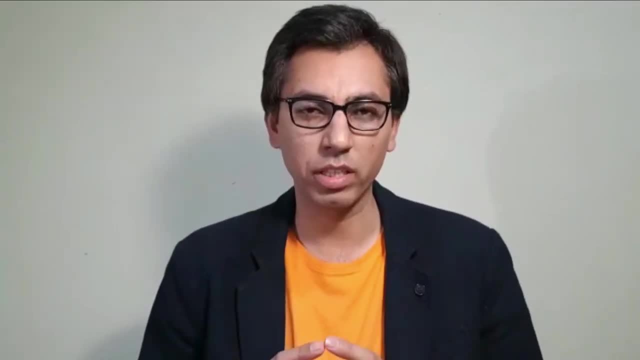 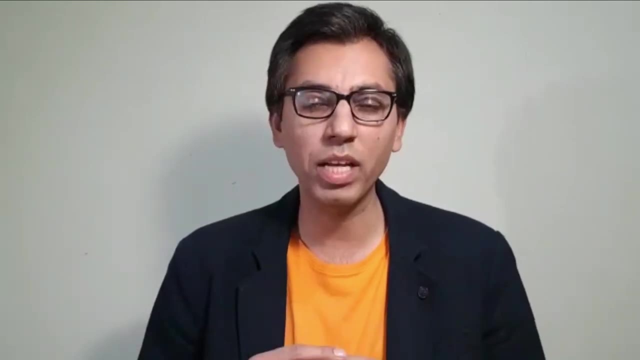 projects, so stay tuned. if you are working on a project or you are managing a project, there might be range of questions that you have come across. those questions could be like: will the project be finished under the budget? will the project will be finished before the schedule? will the? 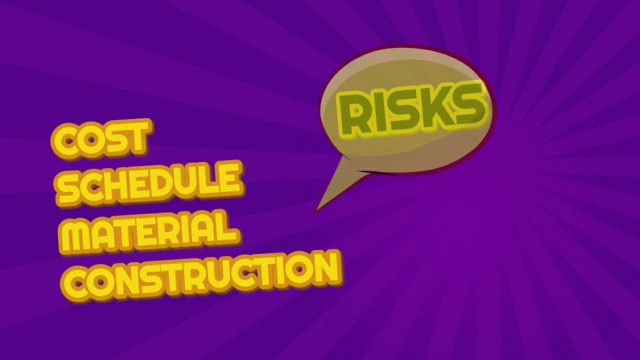 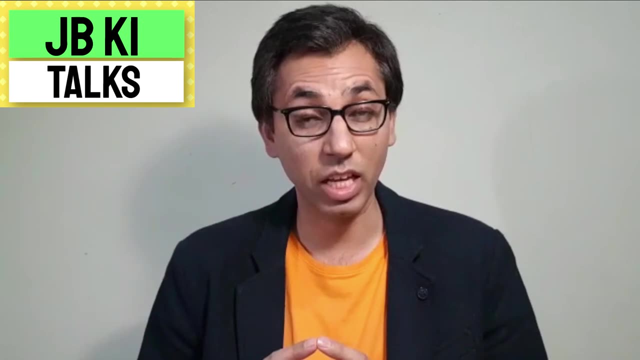 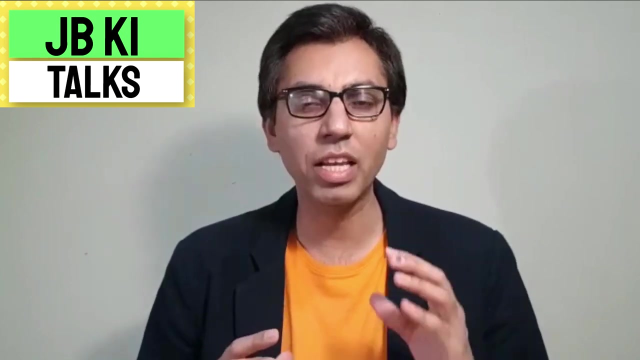 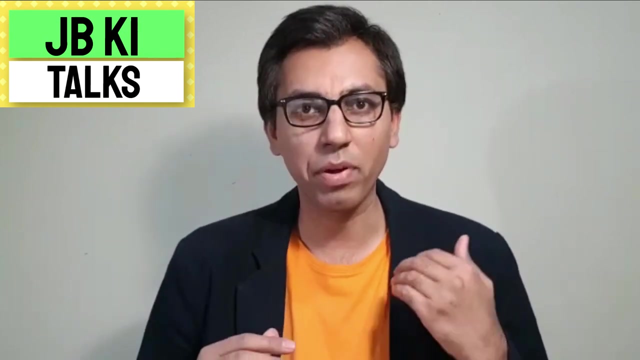 project be completed? what are the potential risks during detailed design construction installation? what could be the procurement issues? there could be a lot of other questions as well. a construction industry survey shows that there are only five percent projects who met the initial estimated cost and budget. if that number, that five percent, is valid, then my previous all questions. 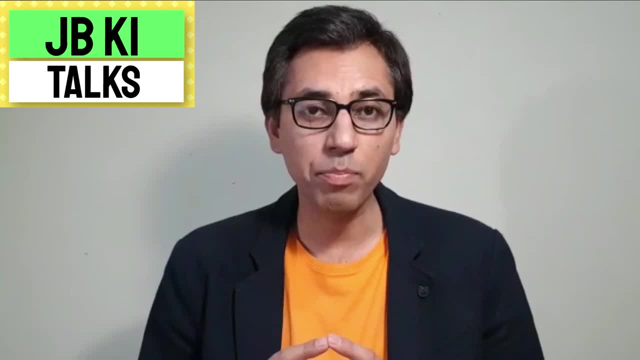 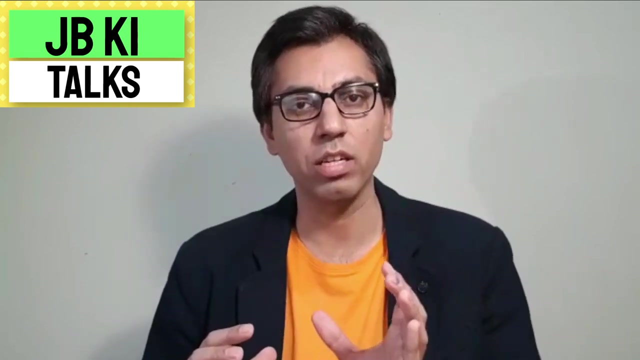 and concerns are valid. to address those questions, the best solution is to invest money, time, efforts in the early in planning stages of any particular project of production life cycle. now i will talk about production life cycle, a typical example, and from there i will tell you where feed front and engineering design falls. now let's talk about 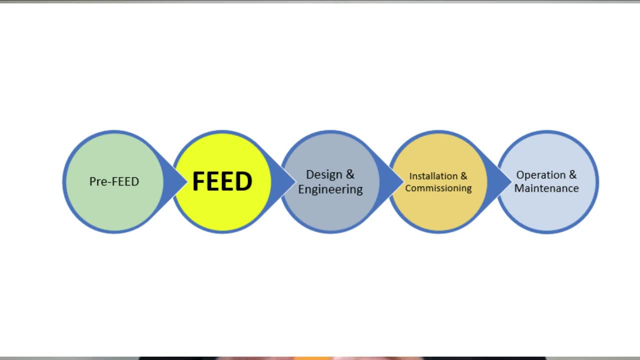 a typical production life cycle. a typical production life cycle has five stages. they are like conceptual study or pre-feed, front-end engineering and design, or feed. third is a design and engineering, fourth is installation and commissioning and fifth is operation and maintenance. now we come to know that feed is a part of early planning for 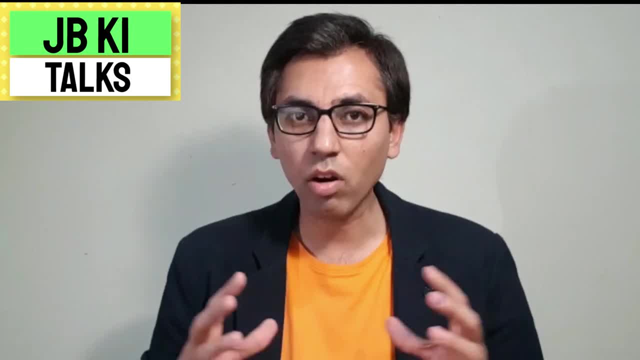 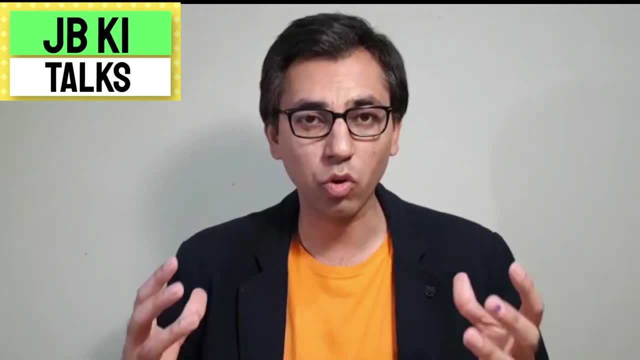 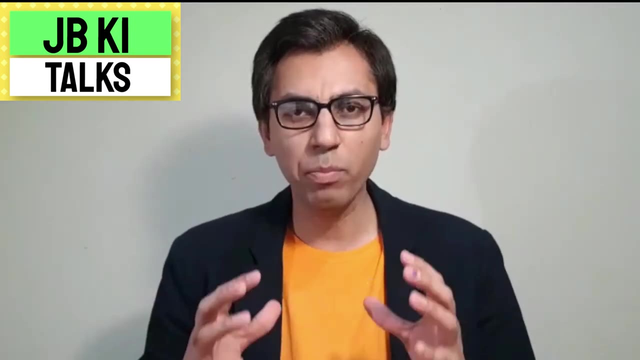 any particular production life cycle. feed does not only give us a cost to make, but it also gives us more than that, like it could be: total scope, schedule, risks and even the project viabilities after feed introduction. now i will briefly explain how a typical feed project is. 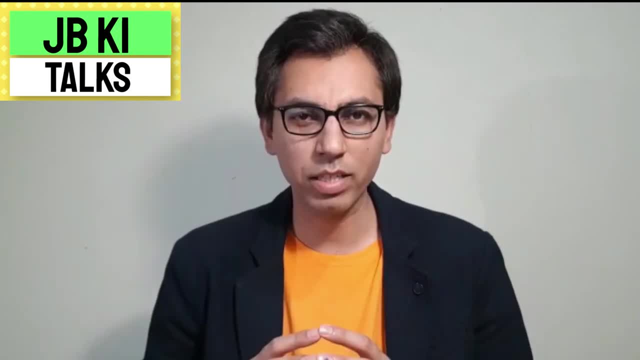 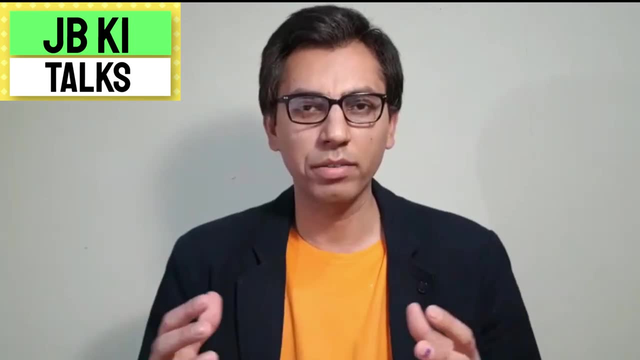 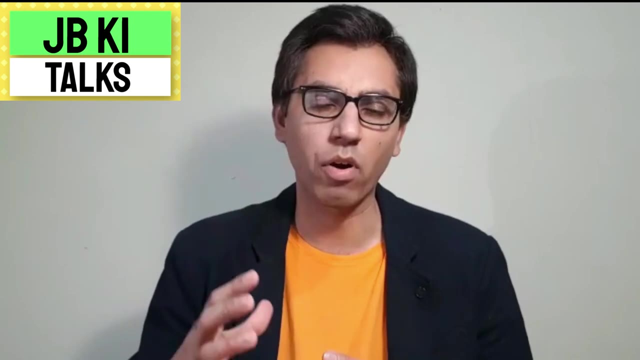 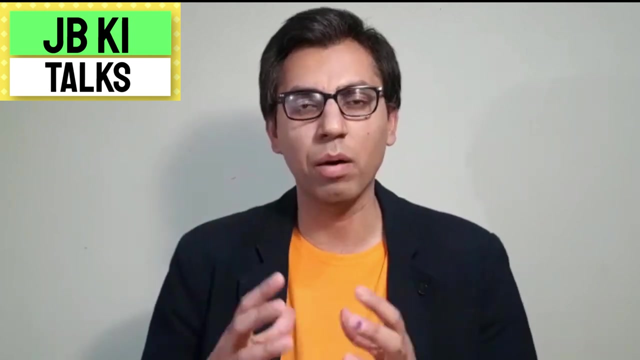 executed. every project and organization is unique but in broader term, a feed project is executed in three steps. step number one: for multiple disciplines project, there is a list of deliverables that we need to produce for that particular project. in step number two, on the basis of deliverables that we produce, we prepare a final outcome of that free project. and in step 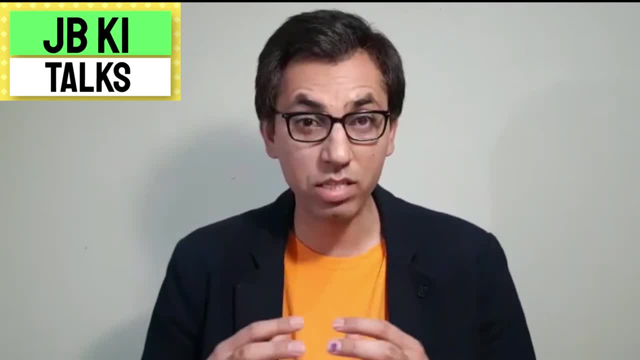 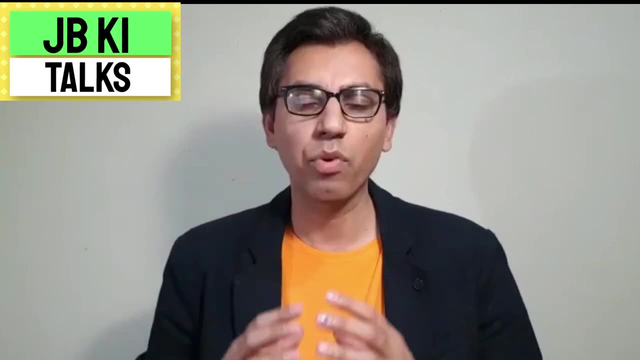 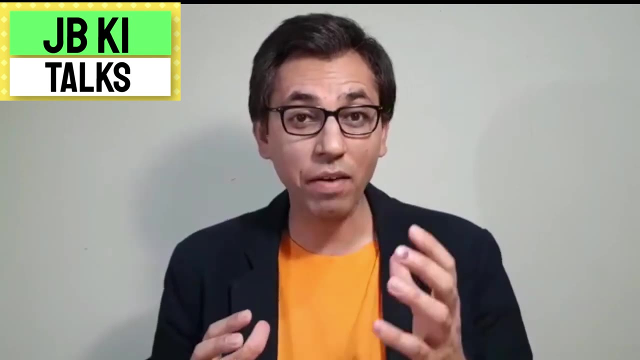 number three, i will share common outcomes or concerns that we can have after the feed conclusion. this example is just for guidelines for your project or for your organization where you are working. this example could vary, so you have to change and you have to make sure that your client expectations 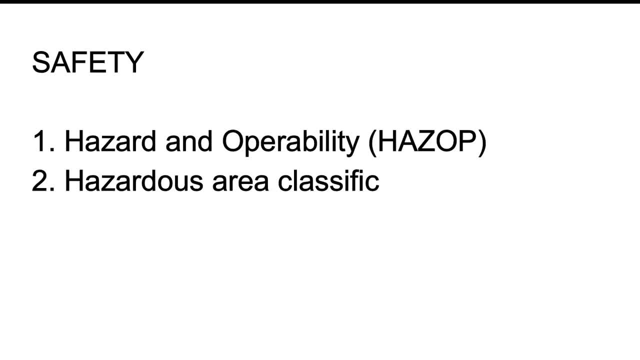 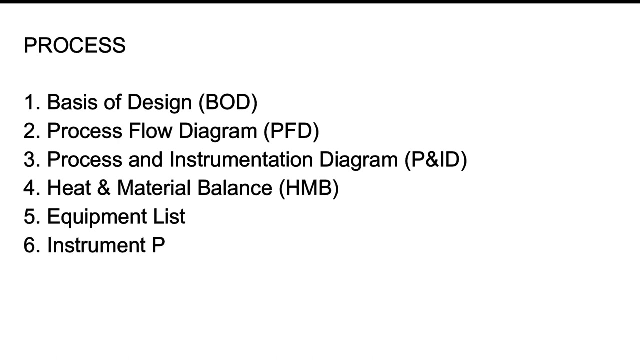 and requirements are met. first for discipline could be safety, and the deliverables could be hazard. hazard and operability, hazardous area classification, safety philosophy, environment, impact assessment. the list of deliverables could be more or less depending on the requirements of the project. now let's see second example of discipline. like process, 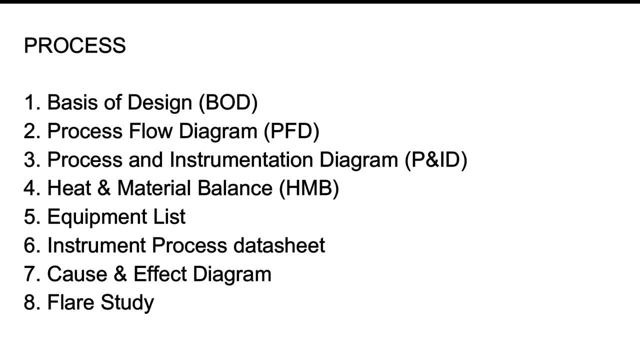 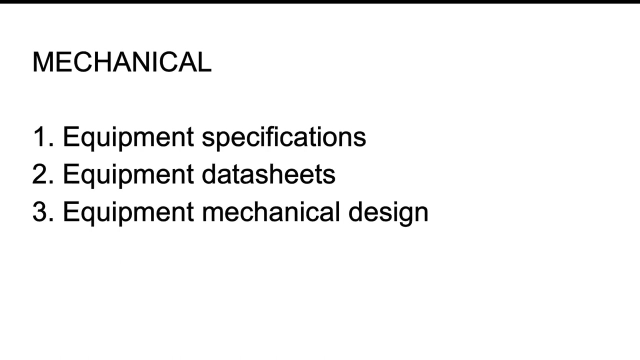 the list of deliverables could be like basis of design, bod process flow diagram, pfd process and instrumentation diagram, pnid, heat and material or mass balance equipment list, instrument process data sheet, causing effect diagram, and could be like flare study- next discipline, mechanical- and the list of deliverables could be like: 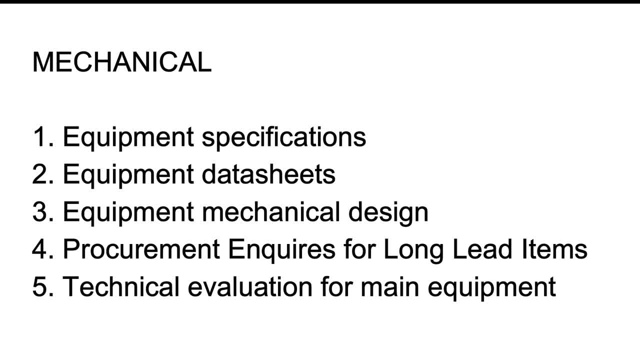 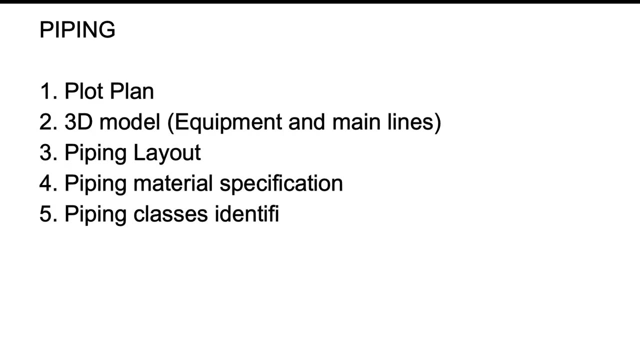 equipment specifications, equipment data sheets, equipment mechanical design. procurement inquiries for long lead items. equipment specifications. equipment specifications, equipment specifications or critical items. technical evaluation for main equipments or items. next discipline example is for piping, and the list of deliverables could be like plot plan 3d model for equipment or for main piping. piping layout, piping material specifications. 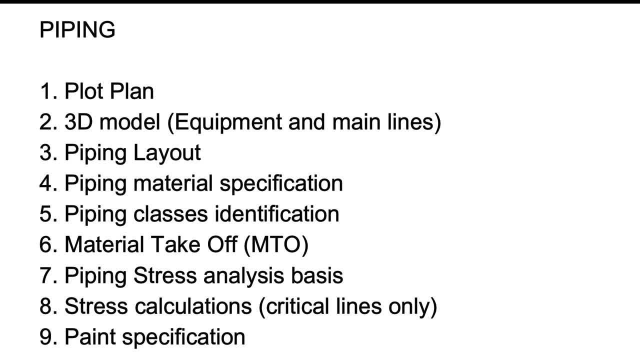 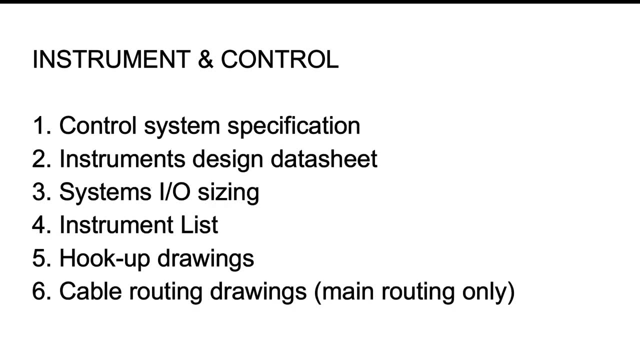 piping class identifications material take off. piping stress analysis, basis, piping stress analysis for critical lines, paint specification, etc. next discipline is instrument and control and the deliverables could be like control system, specification instruments, design data sheet system, input output, sizing instrument. point out of sizing instrument list: hookup drawings, cable routing drawings for main routing. 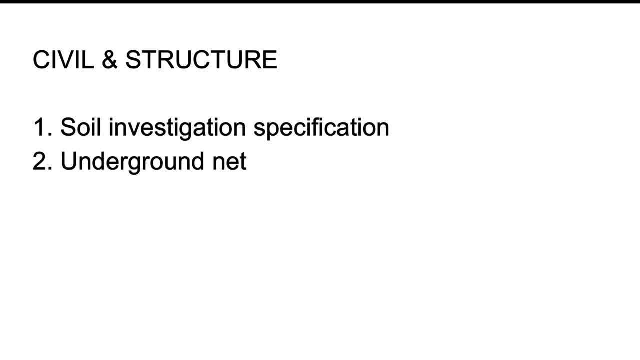 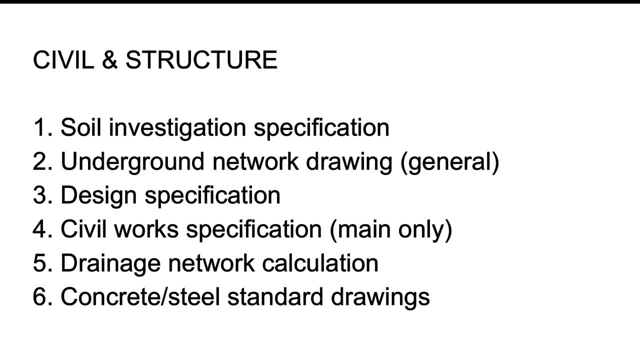 and again the list of deliverables could be more or less depending on the nature of project. next discipline is civil structure and the deliverable examples are like: soil investigation specification. underground network diagram. underground network drawing design specification. civil work specification. drainage network calculation. concrete or steel standard drawings. 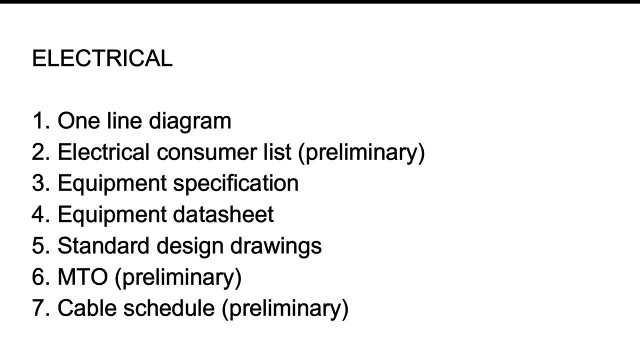 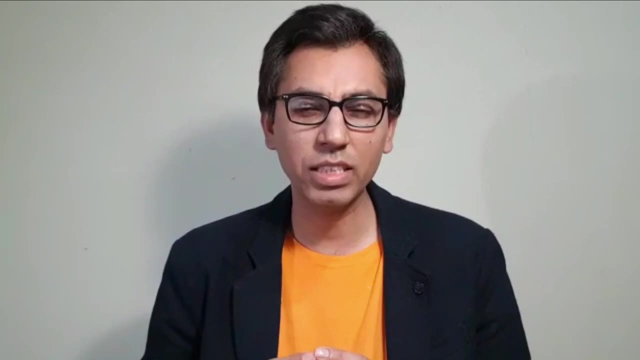 and if there is a discipline electrical involves in that particular project, then deliverables could be like one line diagram. electrical consumer list. preliminary equipment specification, equipment diagram, standard design drawings, mto cable schedule- preliminary. now in step two let's see what are the outcomes or results we should expect to have after the 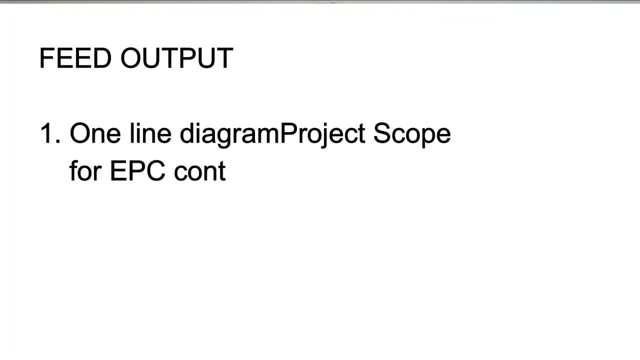 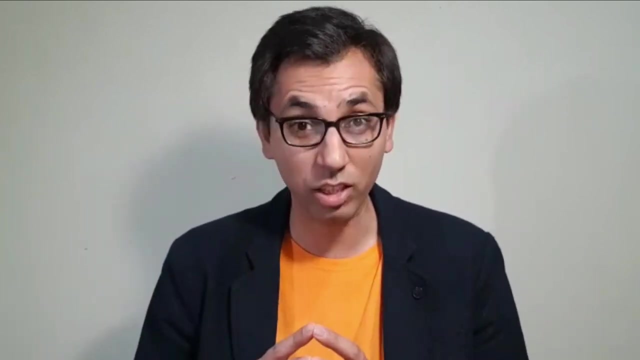 successful field project like it could be: project scope for epc, contractor, overall project cost estimate, procurement estimates and could be project schedule. now, in step three, i will share a few of the common outcomes or concerns that we can see after successful field project. they could be like: 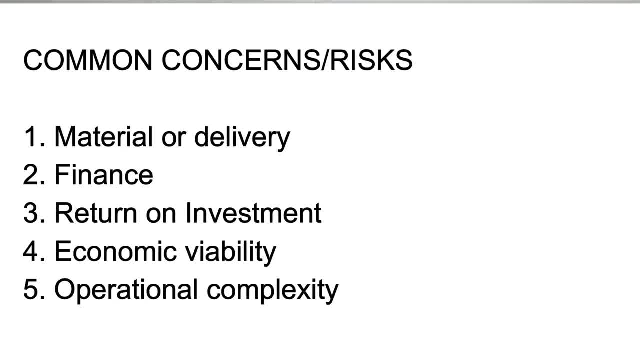 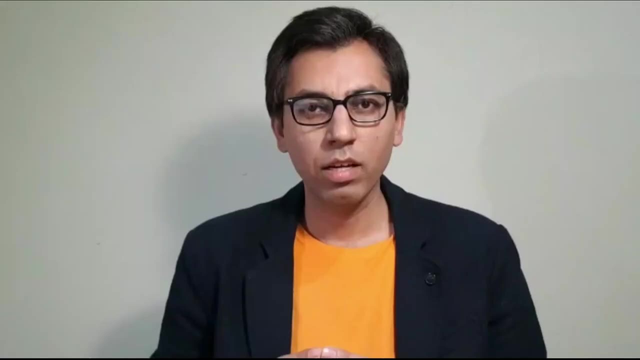 concerns about material or equipment delivery, availability of finance. if there is any social or political impact of the project, we should be able to know about return on investment and that could lead to economical viability, and we should know if there is any operational complexity. now, at the end of this video, I want to summarize field front-end engineering.